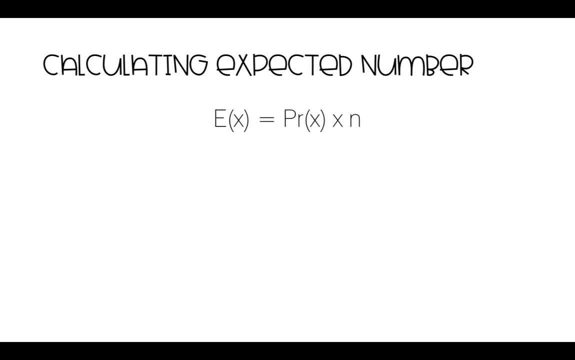 number is us working out. well, if we get this probability so far and we multiply it by how many numbers there are or how many times we do the experiment, that will give us our expected number. So probability we know to be. you know the number of successful trials over. 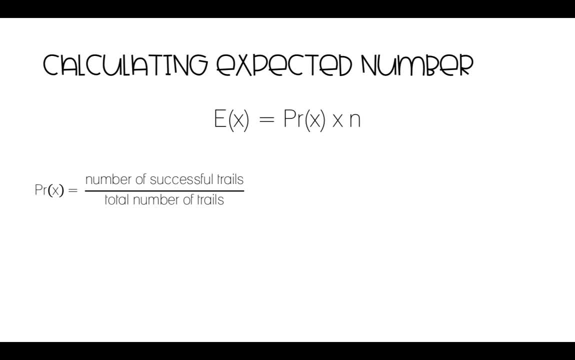 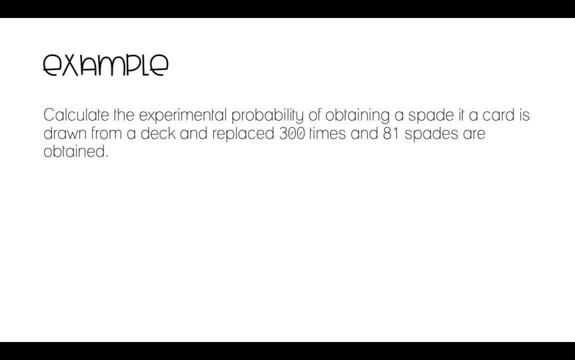 how many trials we completed, and n is the number of trials, so how many times we complete the experiment. Now let's do an example, So calculate the experimental probability of an event. So we're going to use our probability of obtaining a spade in a if a card is drawn from a deck and replaced. 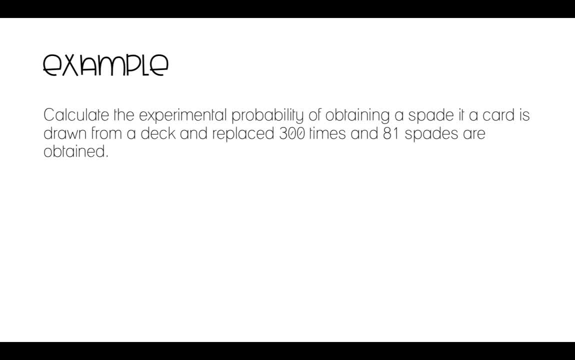 300 times and 81 spades are obtained. So we know how many spades we're getting and we know how many times we're doing the experiment. So what we do is we say: the probability equals the number of successful trials. so how many times we get a spade over the number of times we completed the 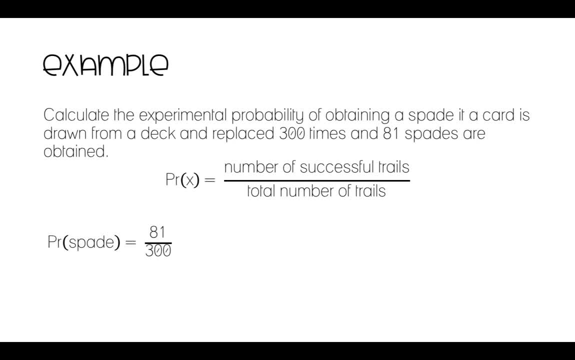 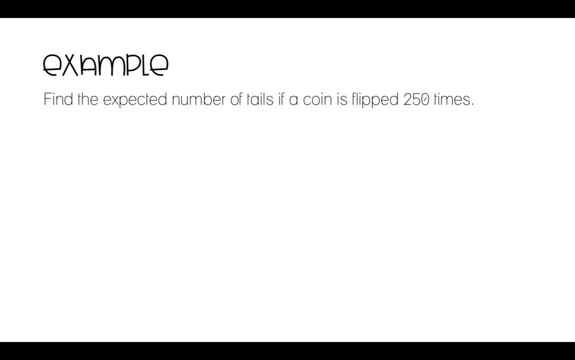 experiment. So probability here equals 81 over 300.. That's the experimental probability that we've, which gives us 27 over 100. okay, let's find the expected number of tails if a coin is flipped 250 times. so expected number gives us means we use the. 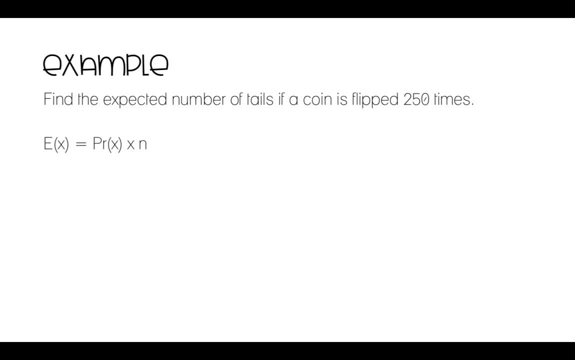 probability times n. so the probability would be: well, there's one chance of us getting a tail every time we flip a coin out of two possible outcomes. so we do the expected. the probability of tails is one half, and so the expected number of tails would be 1 half times 250, which would give us 125. so what we're saying. 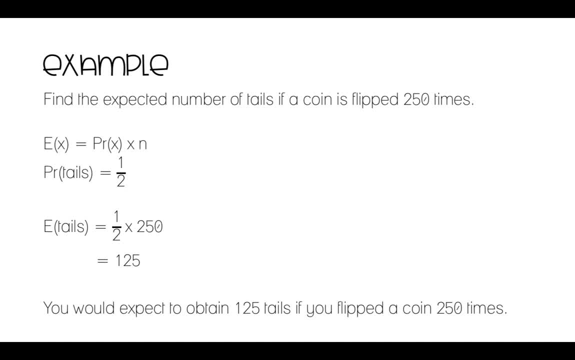 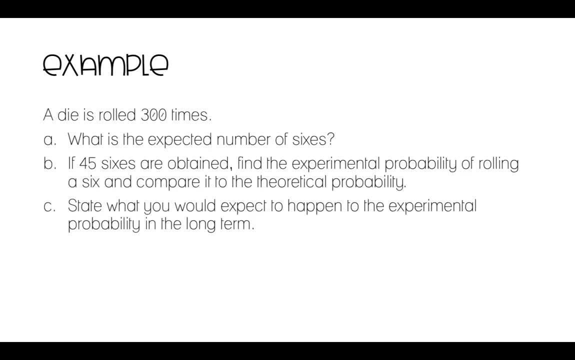 here is: we expect to obtain 125 tails. if you flipped a coin 250 times- now let's do a multiple step examples. so a dies rolled 300 times, what is the probability of tails being flipped twice? is the expected number of sixes? okay, that's the first question. if 45, we'll go. we'll go. question. 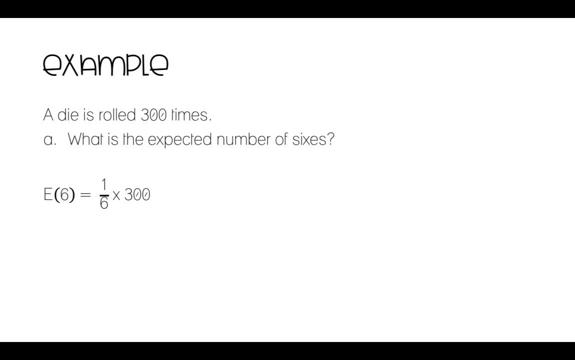 by question. so what is the expected number of sixes? so expected number of sixes equals one sixth, because that's the probability of us getting a six, because there's one six on a dice out of six numbers. so one sixth times 300, which gives us an expected number of 50. so we would expect to get